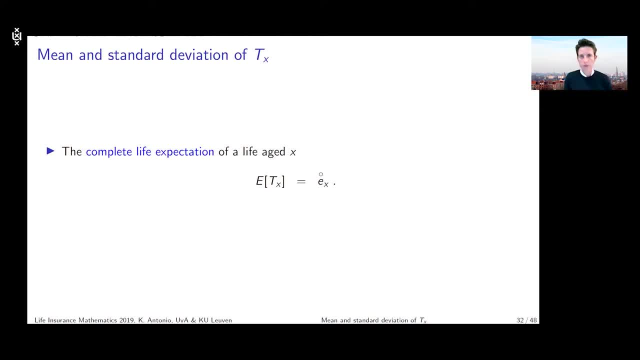 That is referring to the fact that I want to calculate the expected value of the future lifetime of this policyholder of age X. So how are we going to do that? Well, we will be relying once again on our expressions for survival function, force of mortality, and so on. 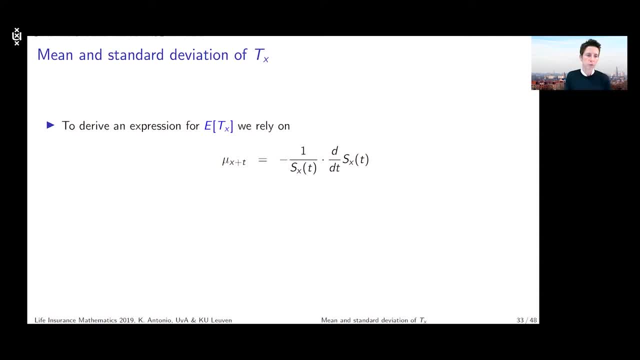 Right. So do remember that we started from this one: the force of mortality for an X plus T year old. We wrote it Earlier on in this particular way. Right Now I know that for an actuary, Now I know that an actuary will rewrite this survival function as X evaluated in T will denote that with the actuarial symbol TPX. 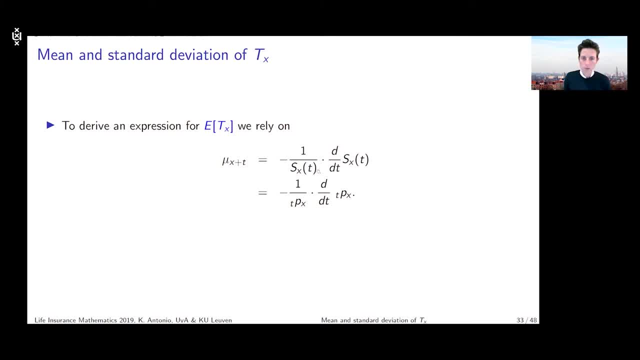 So I can express the same thing using my actuarial notation Right And as a consequence, I retrieve that my density function FX, evaluated in T Right. I can see that as my survival function multiplied with my force of mortality And I can rewrite this product as minus the derivative with respect to T of my TPX. 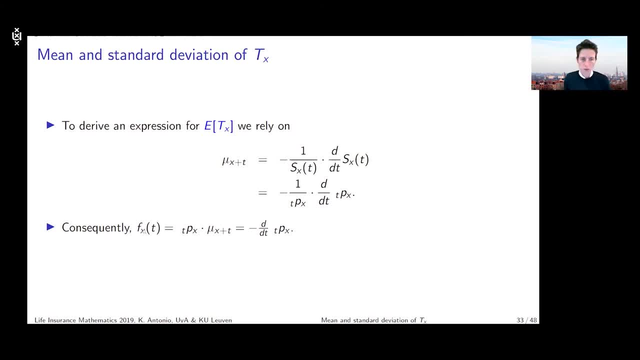 OK, so the connection here between the density function and the force of mortality and the survival function, that's something we did earlier on. And then the next equality follows from the notation over here. So how do I want to use this? So how do I want to use this expression? 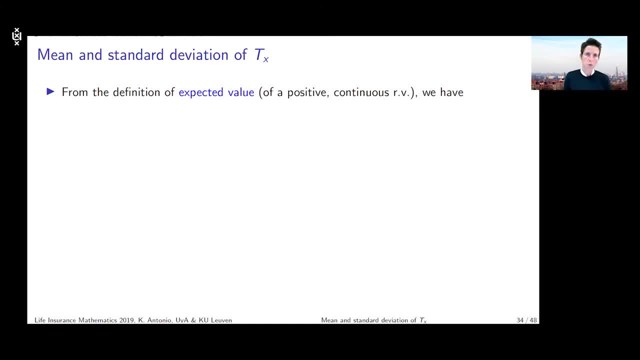 Well, you know from your probability and statistics course that to calculate the expected value of a positive continuous random variable, you can start as follows: You're going to take the integral from zero to plus infinity of all the of the outcomes that your variable can take, multiplied with the PDF of the variable evaluated in these outcomes. 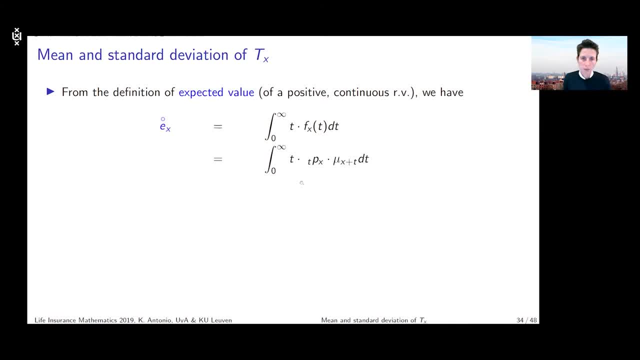 T. So this is a very general definition. In the next step, I'm going to replace my PDF with my survival function, TPX multiplied with my force of mortality, the mu X plus T, And I know from the previous sheet that I can rewrite this product, TPX, mu X plus T, as minus, the derivative of my survival function.